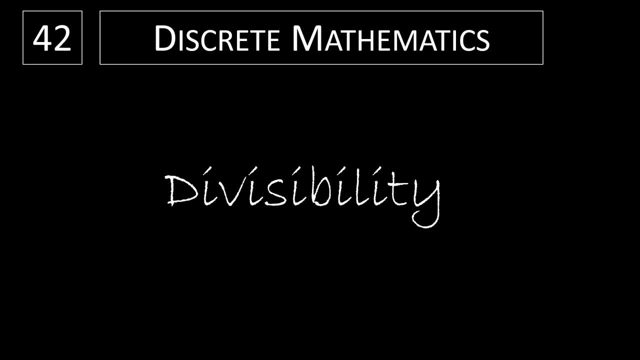 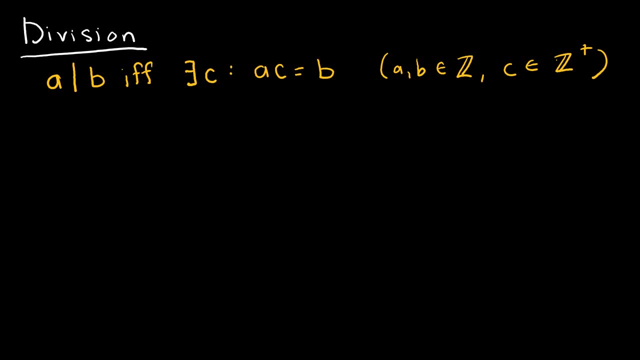 In this video we're going to discuss divisibility, So I want to introduce some new notation to you and that is the divides notation, and that's right here. So this says: a divides b if, and only if, there exists some value c, such that a times c is equal to b and c is a positive integer. So a and b are 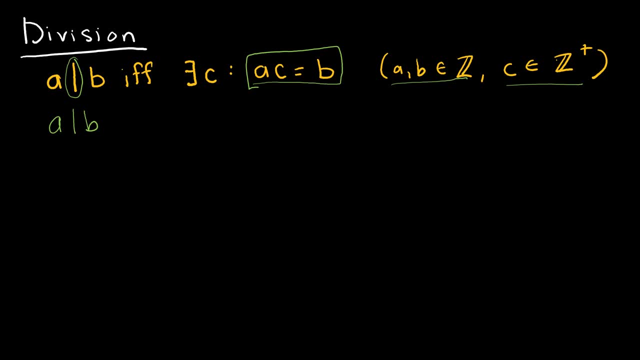 integers. c is a positive integer. So if I had a question like 3 divides 15.. 3 divides 15 tells me 3 times some number, c should equal 15.. If I divide each side by 3, I get c is equal to 5.. Therefore, 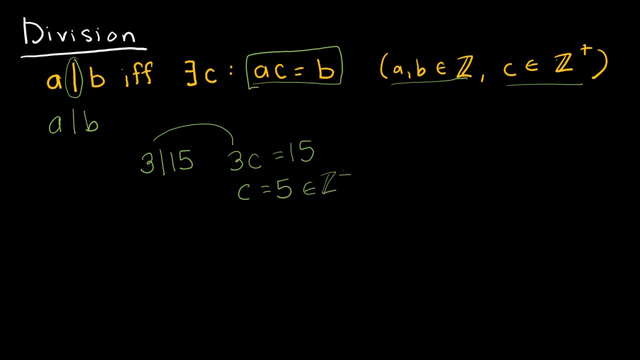 since 5 is in fact a positive integer, I can say that this is true, that 3 does divide 15.. So essentially we're just saying: does that number go into a positive integer? So if I had a question like: 3 divides 15, tells me 3 times some number c. 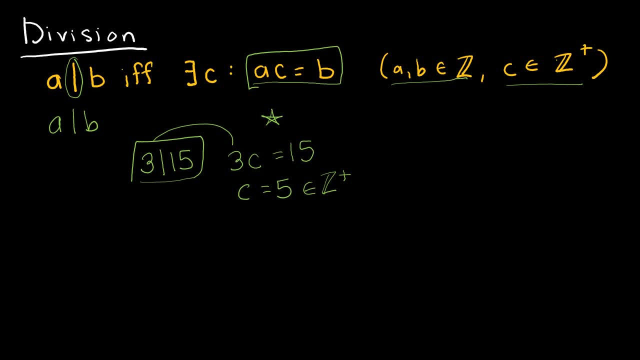 equals 15.. So you can do all of this math over here, but you're far along enough in mathematics that a lot of these you can do in your head. But it's important to understand the process, because I'm going to give you, obviously, things that you cannot do in your head or things that 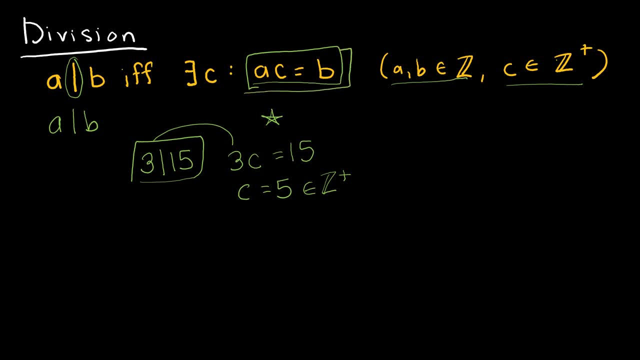 you'll have to use in proofs. So this would be a prime example of something that I might have to substitute for in a proof. Say I had 3 divides 22. Again, using this definition, I can say: 3 times C equals 22.. Dividing each side by 3, I get C equals 22 thirds. 22 thirds certainly. 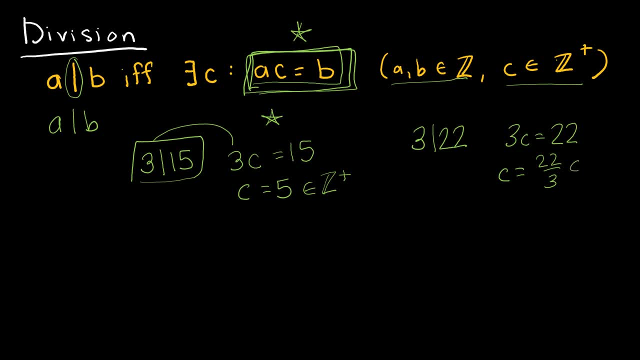 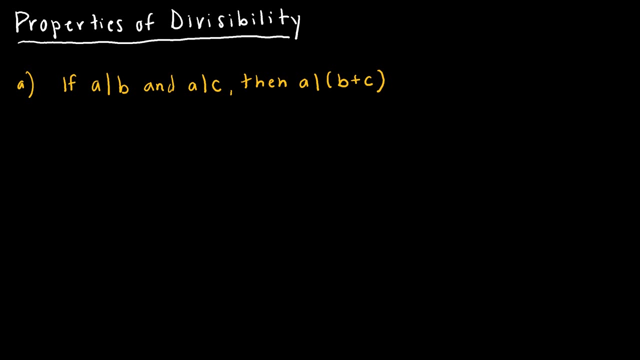 makes the equation 3 times C equals 22, true, However, since this is not a positive integer, then this is not divisible, So notice the notation change. Let's take a look at a few properties of divisibility and also their proofs, because 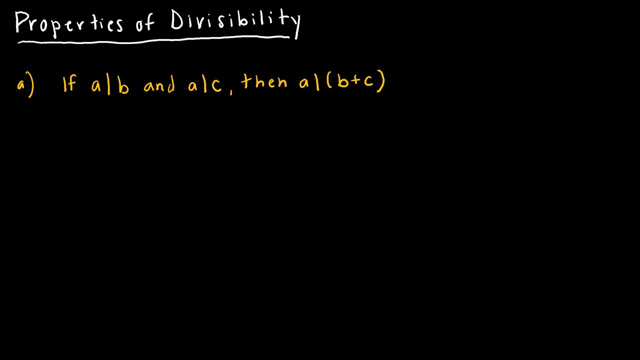 obviously I can tell you a property is true, but you'll want to actually prove it's true Before we prove it. let's just look at an example We have here. if A divides B, so let's say 3 divides 15, and A divides C, let's just use 6 because obviously 3 goes into 15, 3 goes into 6.. Then it tells me that A divides B. so let's say 3 divides 15, and A divides C. let's just use 6, let's just use 6, because obviously 3 goes into 15,, 3 goes into 6.. Then it tells me that A 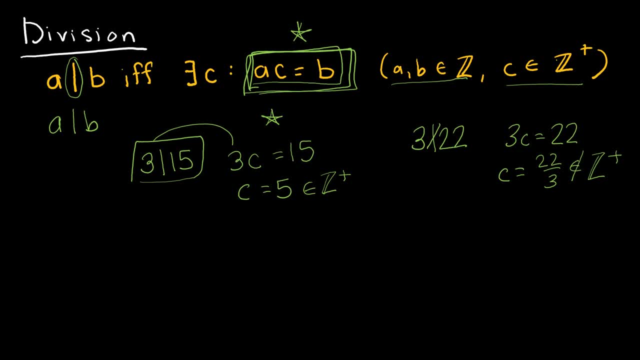 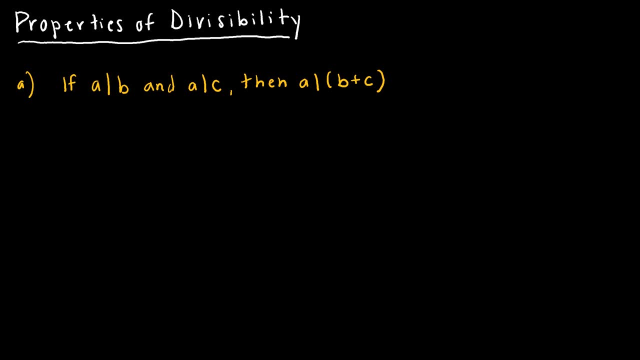 then this is not divisible. So notice the notation change. Let's take a look at a few properties of divisibility and also their proofs, because obviously I can tell you a property is true, but you'll want to actually prove it's true. 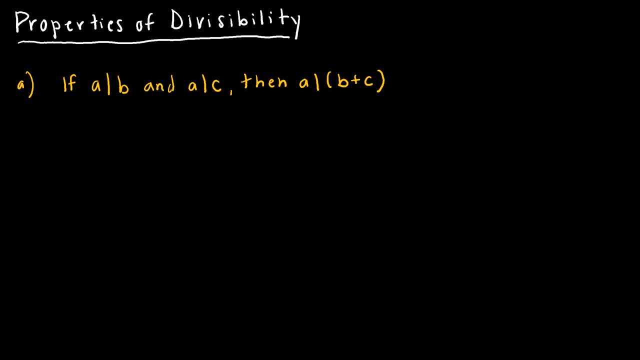 Before we prove it, let's just look at an example We have here. if A divides B, so let's say 3 divides 15, and A divides C, let's just use 6, because obviously 3 goes into 15,, 3 goes into 6.. Then it tells me that A divides B. so let's say 3 divides 15, and A divides C. let's just use 6, let's just use 6, because obviously 3 goes into 15,, 3 goes into 6.. Then it tells me that A 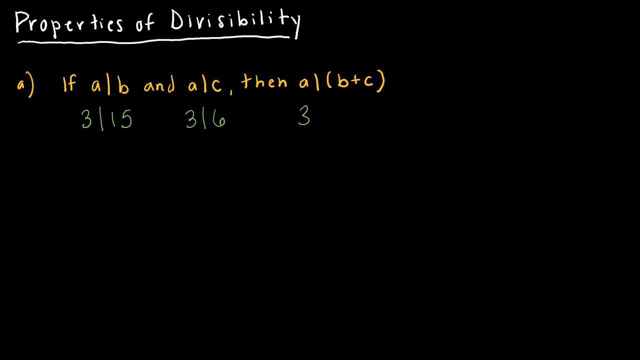 A divides B plus C, so 15 plus 6, which is 3 divides 21.. So, yes, I've shown it's true for the value of 3, and that's all I've done. Now, of course, what we would want to do is to be able. 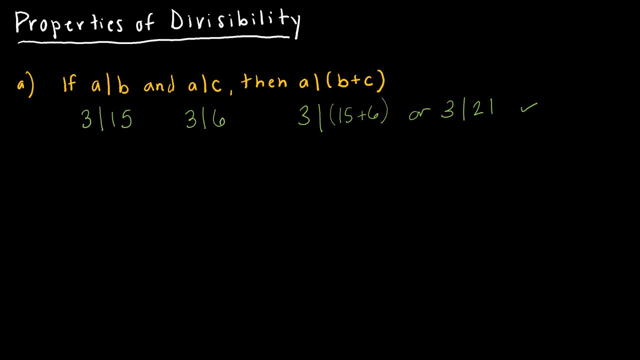 to prove it is true for all integers, and that's what we're going to do now. Now, whenever you're doing a proof, keep in mind that you're always going to be looking at the value of 3, and that's a definition, things that we already know. And so what do I already know? I know that A divides B. 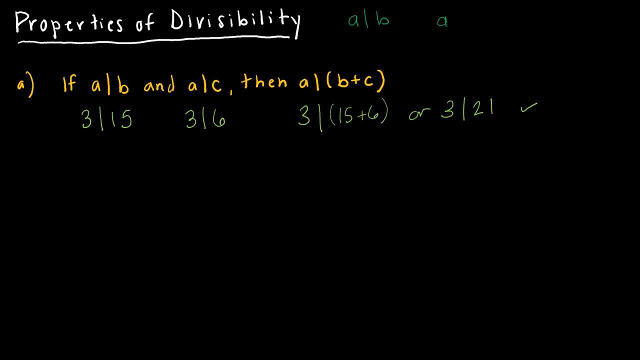 tells me that A times C is equal to B for some value of C. Now that might get a little bit confusing, because, notice, I've got a C here in my question that I'm going to prove, and so instead of using C, I'm going to use some other variable, S, or I'm also 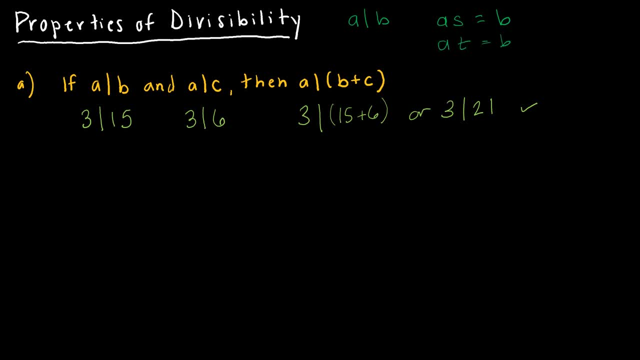 going to use C, and so, instead of using C, I'm going to use some other variable, S, or I'm also going to end up using T, And so let's take a look at what I mean by that. To start my proof, I'm going to say: there exists. 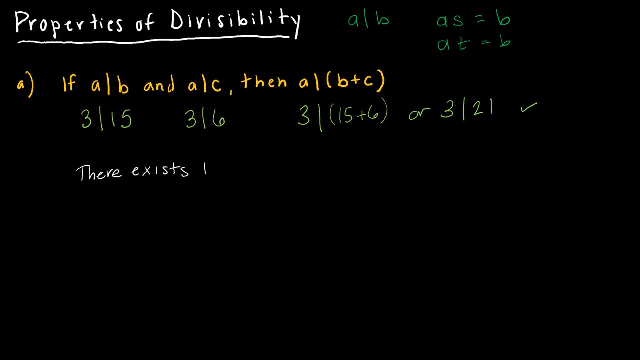 two integers, S and T, And again, I'm just using those because they're not A, B or C, So you can use whatever letters you know bring warmth and joy to your heart. I'm going to use S and T such that. 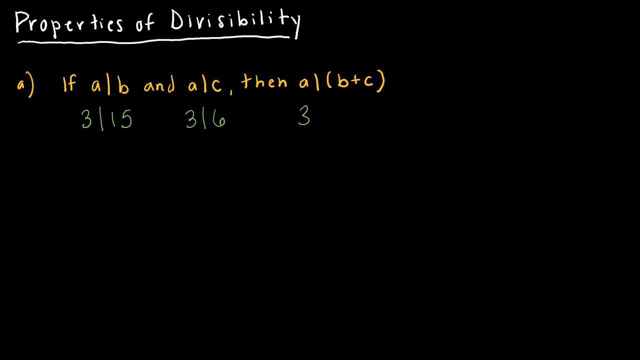 A divides B plus C, so 15 plus 6, which is 3 divides 21.. So, yes, I've shown it's true for the value of 3, and that's all I've done. Now, of course, what we would want to do is to be able. 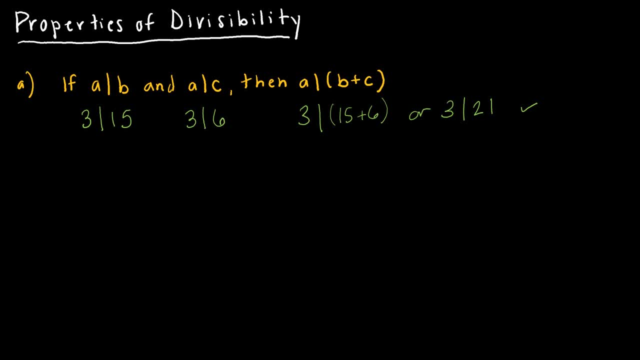 to prove it is true for all integers, and that's what we're going to do now. Now, whenever you're doing a proof, keep in mind that you're always going to be looking at a definition, things that we already know. And so what do I already know? I know that A divides B. 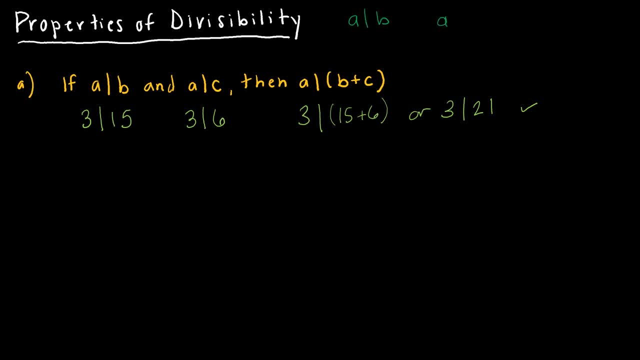 tells me that A times C is equal to B for some value of C. Now that might get a little bit confusing because, notice, I've got a C here in my question that I'm going to prove, And so instead of using C, I'm going to use some other variable, S. 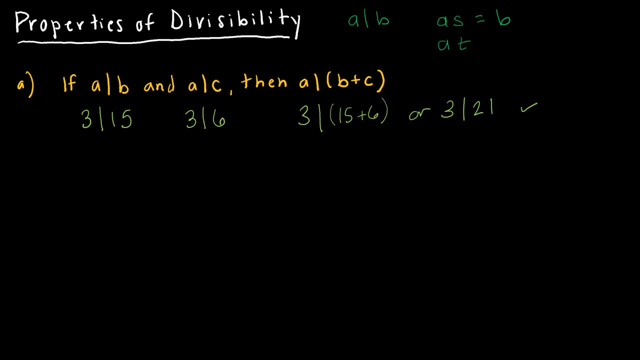 or I'm also going to end up using T, And so let's take a look at what I mean by that. To start my proof, I'm going to say there exists two integers, S and T, And again I'm just using those because they're not A, B or C, So you can. 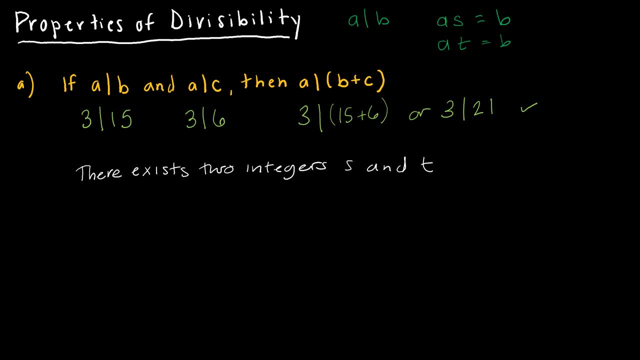 use whatever letters you know bring warmth and joy to your heart. I'm going to use S and T, Such that, And then, of course, I'm going to go back to what I know up here, which is the definition. 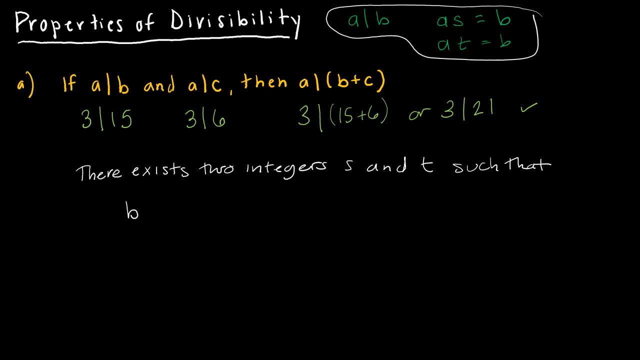 I'm going to say that B, So I'm taking this one first. B is equal to A times S, And then C. So I'm going to change this guy to C. And C is equal to A times T. So I'm going to say that B is equal to A times S, And then C. 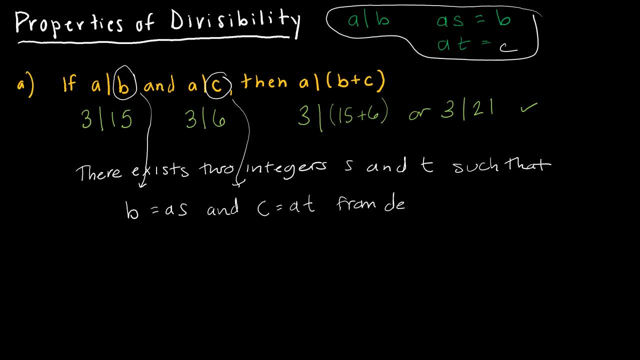 So I'm going to change this guy to C, And then C From definition of divisibility. So not a bad idea to throw in. hey, here's how I know that's true, But I do know that to be true by the definition of divisibility. And then where would I go from? 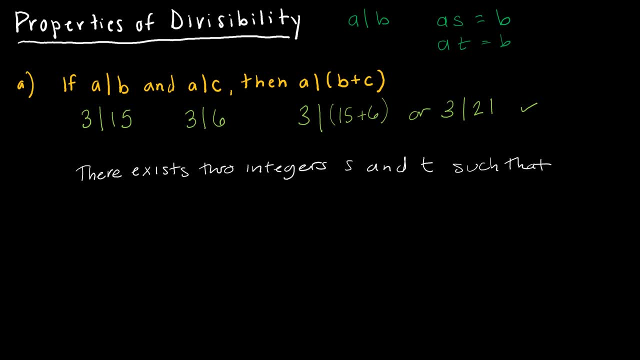 they're not A, B or C, And then, of course, I'm going to go back to what I know up here, which is the definition. I'm going to say that B- so I'm taking this one first- B is equal to A times S. 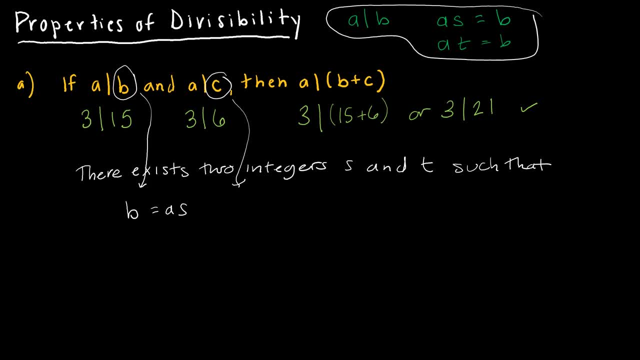 and then C. so I'm going to change this guy to C. and C is equal to A times T From definition of divisibility, So not a bad idea to throw in. hey, here's how I know that's true, But I do know that to be true by the definition of divisibility. 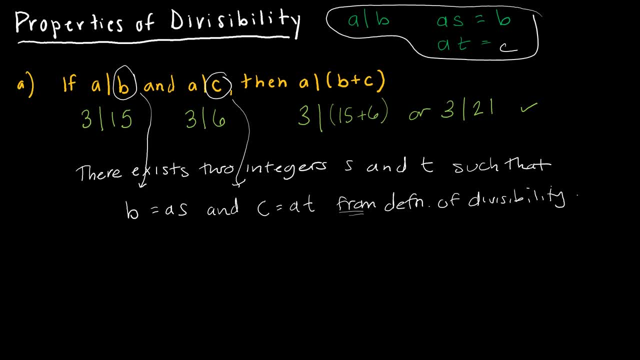 And then where would I go from there? Well, now I'm looking at this statement. This is what I'm trying to prove. I need to show that A now divides B plus C. So let's take a look at B plus C. 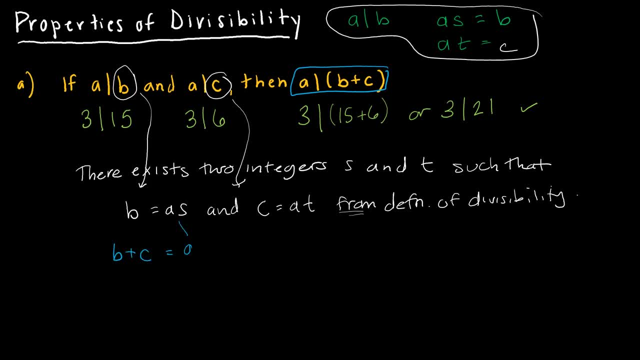 B plus C can be rewritten by substitution as A S plus A T, which, by the distributive property, can be rewritten as A times S plus T. Now I want you to take a look at what I have. I have something in the proper format: A times some value is equal to some other value, So A times S plus T. 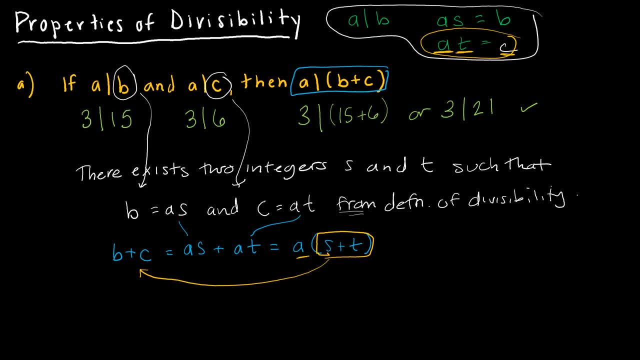 is equal to B plus C. What does that tell me? By the definition of divisibility, it tells me that obviously I can write, and let me just clarify here: b plus c is equal to a times s plus t, and again that's in the proper format. and so that tells me that a I should put therefore: a divides b plus c. 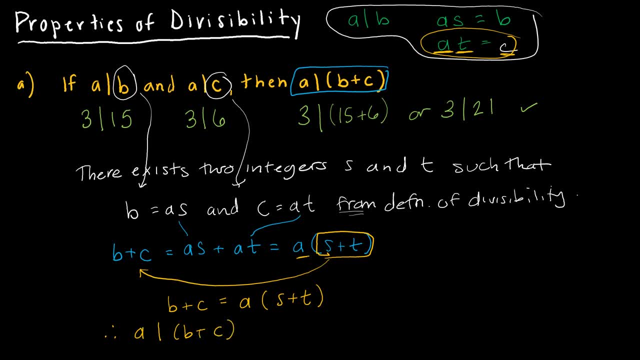 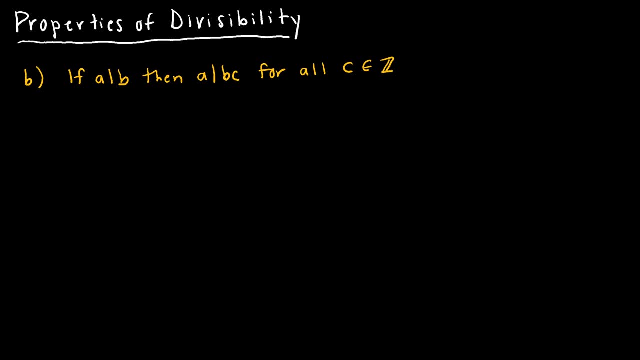 So that is a proof for all values that are integers. Let's look at another property of divisibility. This one says: if a divides b, then a divides b times c for all values of c. So again, before you do a proof, make it make sense in your head. 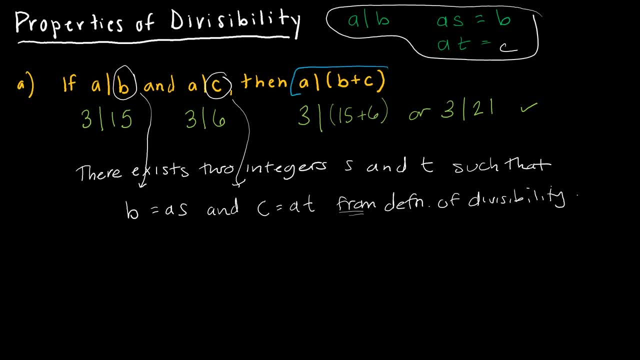 there. Well, now I'm looking at this statement. This is what I'm trying to prove. I need to show that A now divides B plus C. So I'm going to show that A now divides B plus C. So let's take a look at B plus C. B plus C can be rewritten by substitution as AS plus AT. 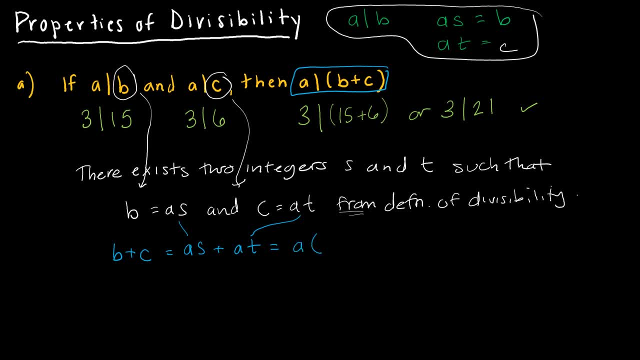 which, by the distributive property, can be rewritten as A times S plus T. Now I want you to take a look at what I have. I have something in the proper format: A times some value is equal to some other value, So A times S plus T. 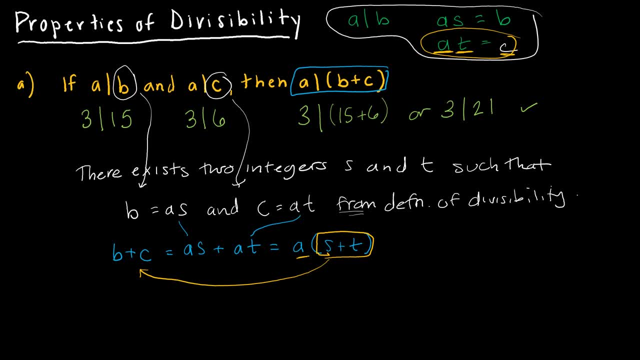 is equal to B plus C. What does that tell me? By the definition of divisibility, it tells me that obviously I can write, and let me just clarify here: B plus C is equal to A times S plus T, And again that's in the proper format. And so that tells me that A: 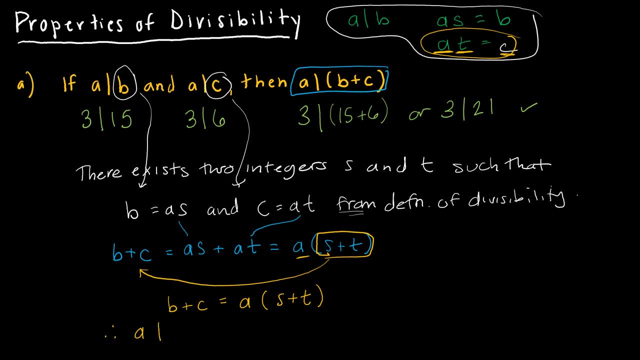 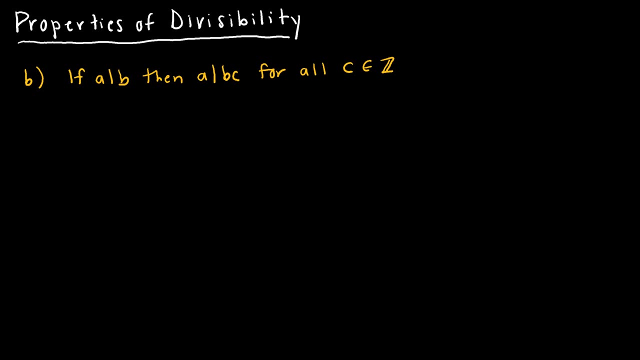 I should put: therefore, A divides C. So that is a proof for all values that are integers. Let's look at another property of divisibility. This one says: if A divides B, then A divides B times C for all values of C. So again, 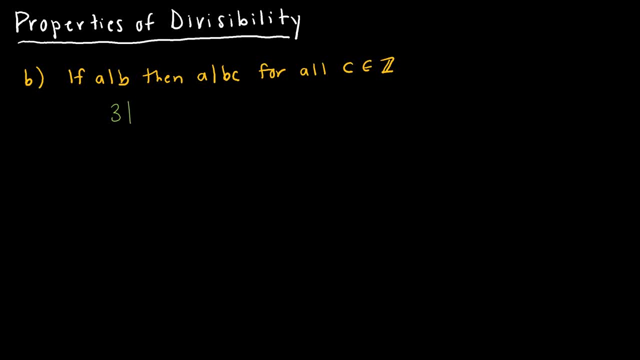 before you do a proof, make it make sense in your head. If 3 divides 15, then 3 divides, say, 15 times 2.. Or 3 divides 15 times 3.. Oops And again. I could continue showing all of these. 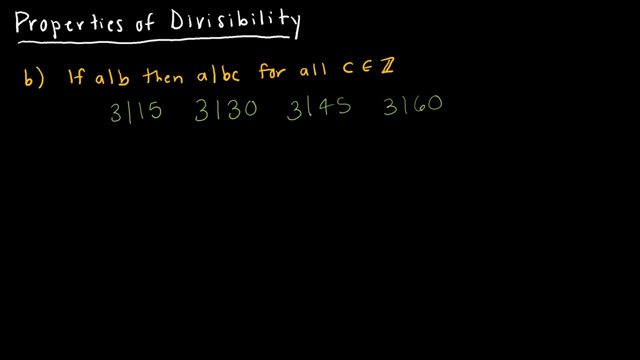 multiples of 15. that 3 goes into. but it only works if I have a proof. So the proof is going to tell me for all values of A and B and C that are integers. So how am I going to go about that? 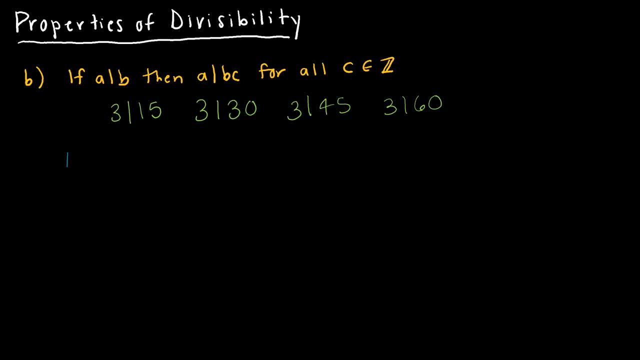 I'm going to start the same way I started on the last one. I'm going to say: if A divides B, then I'm going to use the definition of division to say that B is equal to A times. Now I'm not going to use C again because I already have C in my question. 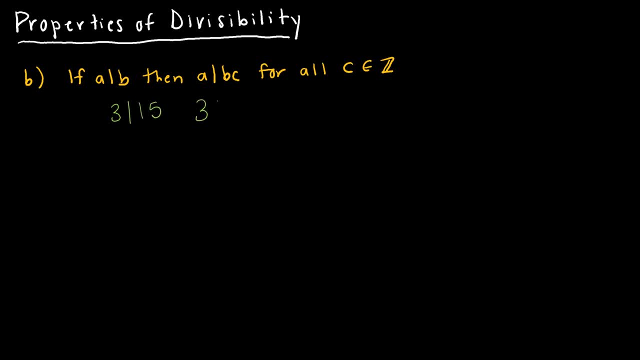 If 3 divides 15, then 3 divides, say, 15 times 2,, or 3 divides 15 times 3.. And again I could continue showing all of these multiples of 15 that 3 goes into. but it only works if I have a proof. 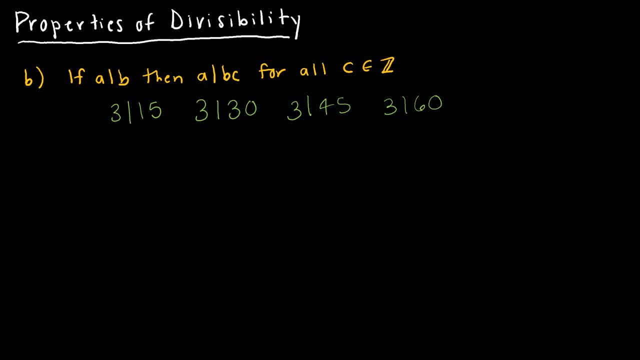 So the proof is going to tell me for all values of a and b and c that are integers. So how am I going to go about that? I'm going to start the same way I started on the last one. I'm going to say, if a divides b, then I'm going to use the. 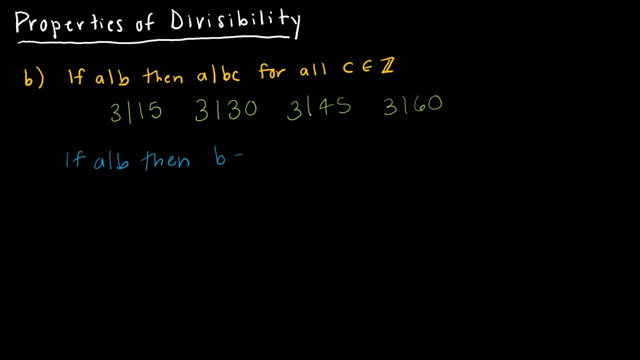 definition of division to say that b is equal to a times. now I'm not going to use c again because I already have c in my question. So I'm going to use t again, as I did before for some integer t. 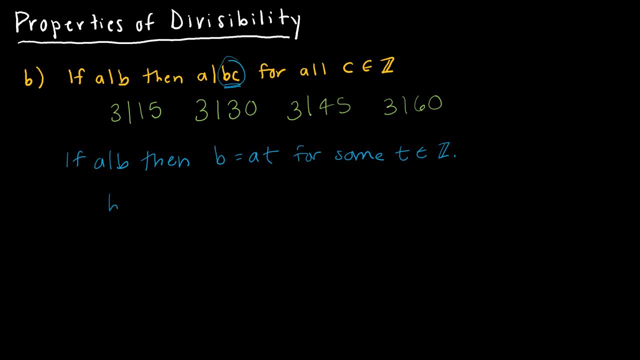 So now I'm going to look at b times c. So b times c is equal to a t times c, And I'm going to say that b is equal to a times c. So I'm just going to regroup that a times tc and of course that's just using the associative property that I can group things differently. 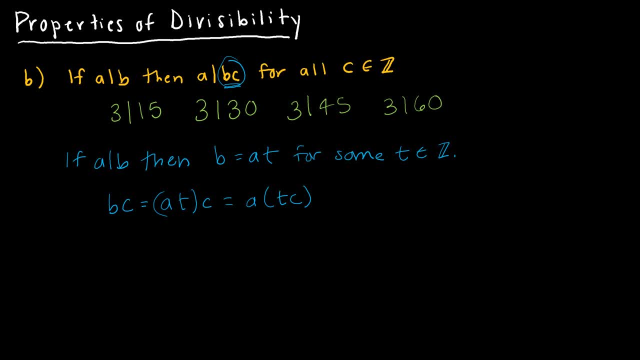 And so the way that it's written. now I can see that a divides bc because again it's written in the proper format: a divides bc by definition of divisibility For our last property. we're saying if a divides b and b divides c, then a divides c. 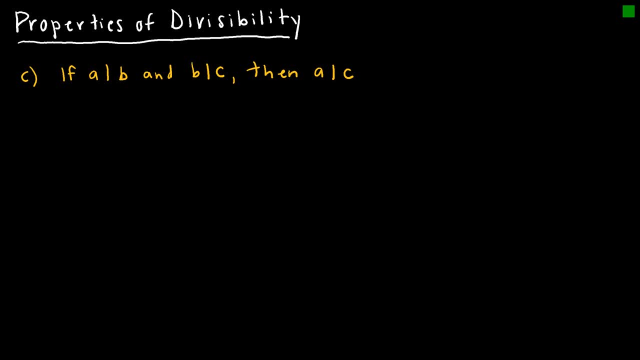 So sort of a transitive property. So here we're saying, let's say 3 divides 6, and 6 divides 18, then 3 divides 18.. So again, yes, we can see this is true. How might we go about proving this? 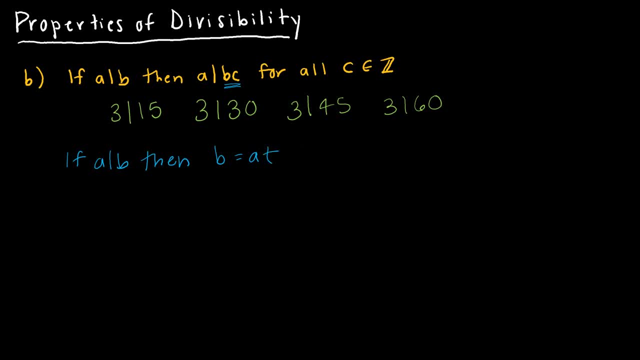 So I'm going to use T again, as I did before for some integer T. So now I'm going to look at B times C. So B times C is equal to 2 times A times C. So if A divides B, then A divides B for all values of C. 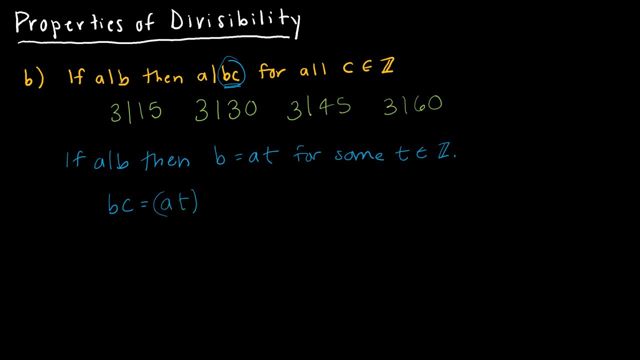 So I'm going to use T again, as I did before, for some integer T equal to AT times C, And I'm just going to regroup that A times TC. And of course that's just using the associative property that I can group things differently. 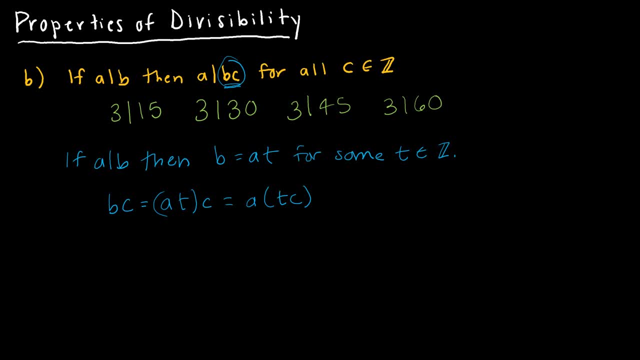 And so the way that it's written. now I can see that A divides BC because again it's written in the proper format. A divides BC by definition of divisibility For our last property. we're saying if A divides B and B divides C, then A divides C, So sort of. 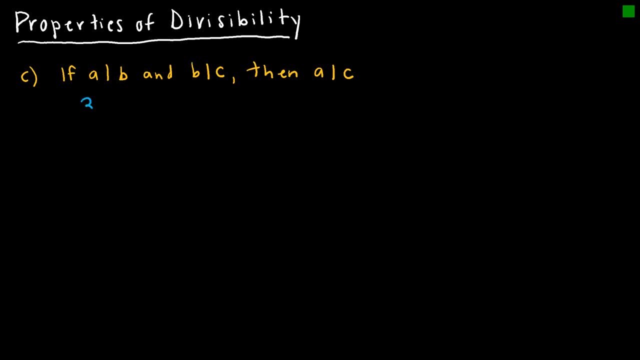 transitive property. So here we're saying, let's say, three divides six And 6 divides 18, then 3 divides 18.. So again, yes, we can see this is true. How might we go about proving this? So we know that since A divides B, again we can look at that definition that says: 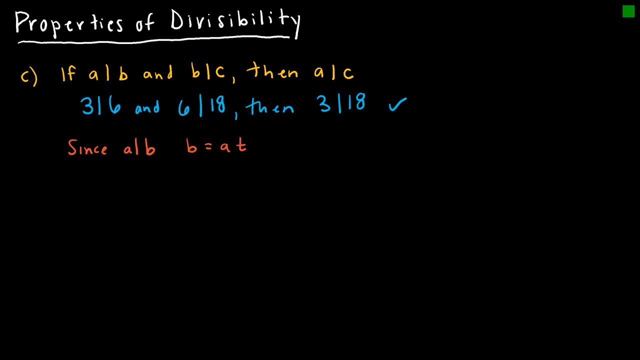 B equals A T. I should have said: then B equals A T for some T. that is an integer. Again, based on that definition, Since B divides C, then C equals B S for some S. that is an integer. So hopefully you can see where we're going with this. So by substitution. 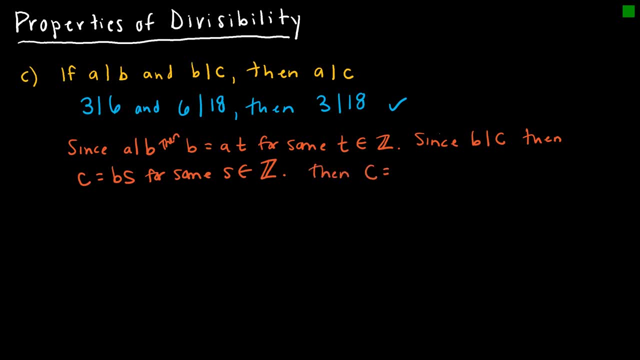 then we can say that C equals, and again, instead of B S I'm substituting A T. Then C is equal to A T times S. And just like we did on that last one, then we could say: or C equals A times S. 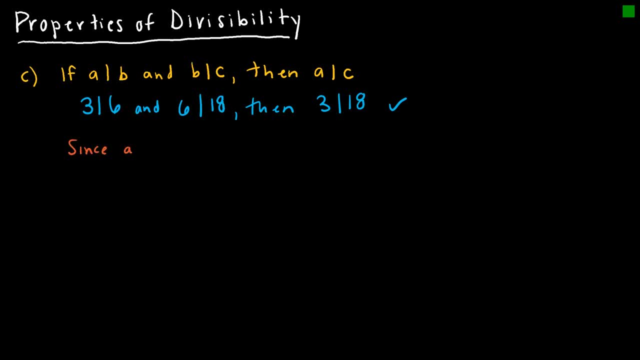 So we know that since a divides b, again we can look at that definition that says b equals a t. I should have said then b equals a t for some t that is an integer, again based on that definition, Since b divides c. 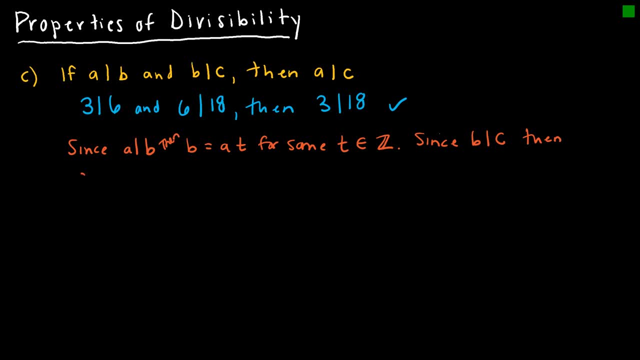 then c equals bs. for some s that is an integer, So hopefully you can see where we're going with this. So by substitution then we can say that c equals and again, instead of bs I'm substituting a t. then c is equal to a t times s. 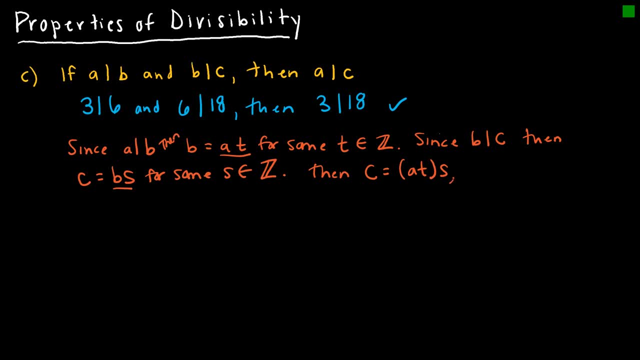 And just like we did on that last one, then we could say: or c equals a times ts, And again, that is just the definition. Therefore, a divides c, And we're all done. Now that we understand divisibility, let's take a look at the definition of divisibility. 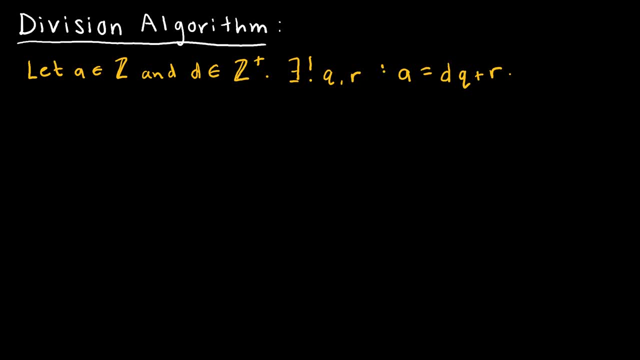 Let's take a look at the division algorithm, which of course has to do with divisibility. Now, just as a reminder, up to this point, if I said something like d divides a, you would say: well, that means a is equal to d times some value c. 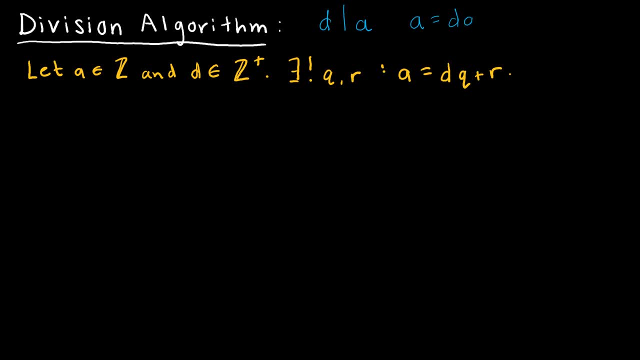 So what we're going to do here in the division algorithm is very similar to that. Instead of c, I'm going to use q because, as we know, it doesn't really matter what variable we use as long as it's not used somewhere else on our question. 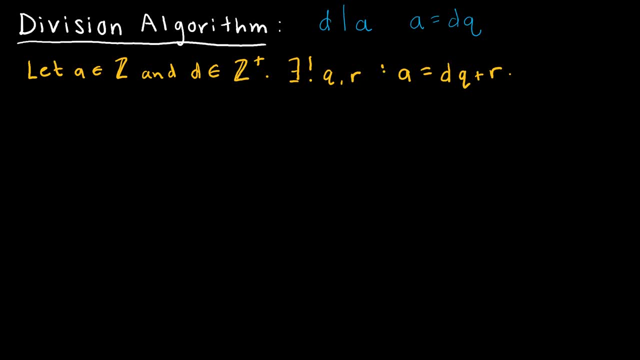 So if d divides a, then a is equal to d times q. The division algorithm says: yeah, that's great, but in the real world sometimes things don't divide evenly and therefore we need this guy, which is a remainder. 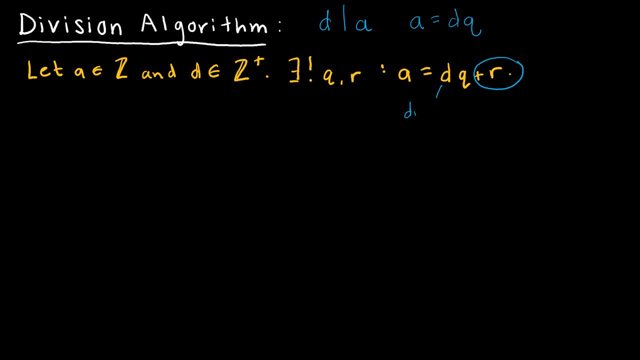 So d is going to represent our divisor, That is, what we are dividing by- q is going to represent our quotient, which is, of course, the answer to a division problem, And r is going to represent a remainder. So let's take a look at an example on how we would use this. 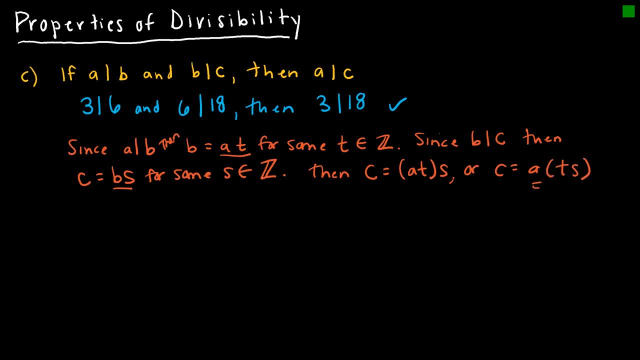 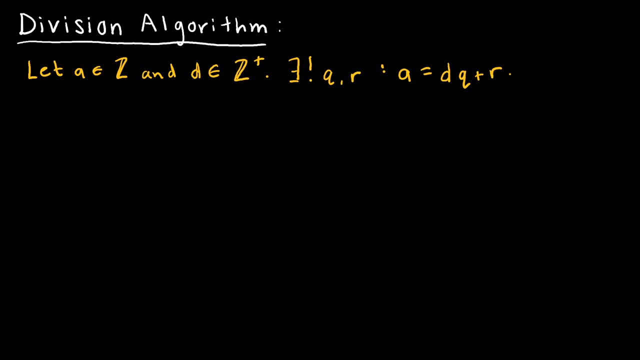 And again, that is just the definition. Therefore, A divides C, and we're all done. Now that we understand divisibility, let's take a look at the division algorithm, which, of course, has to do with divisibility. Now, just as a reminder up to this point, 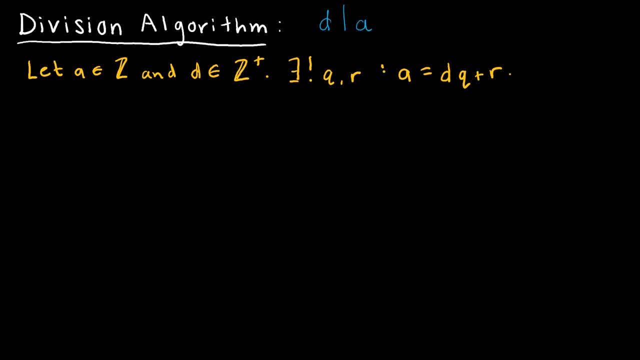 if I said something like D divides A, you would say: well, that means A is equal to D times some value C. So what we're going to do here in the division algorithm is very similar to that. Instead of C, I'm going to use Q because, as we know, it doesn't really. 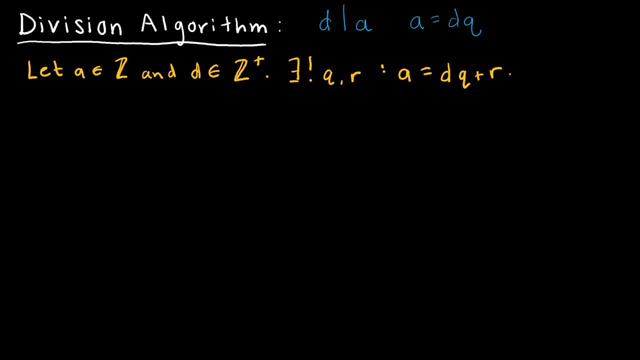 matter what variable we use, as long as it's not used somewhere else on our question. So if D divides A, then A is equal to D times Q. The division algorithm says: yeah, that's great, But in the real world sometimes things don't divide evenly. 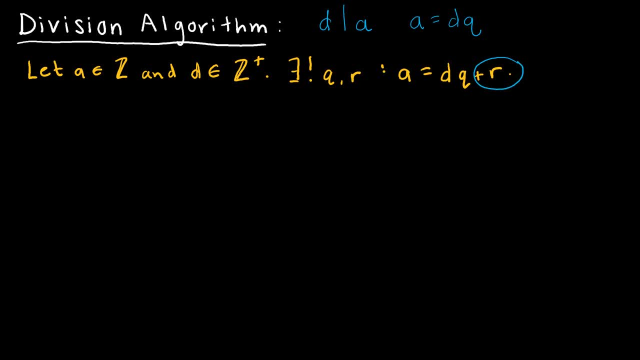 And therefore we need this guy, which is a remainder. So D is going to represent our divisor, That is what we are dividing by. Q is going to represent our quotient, which is, of course, the answer to a division problem. 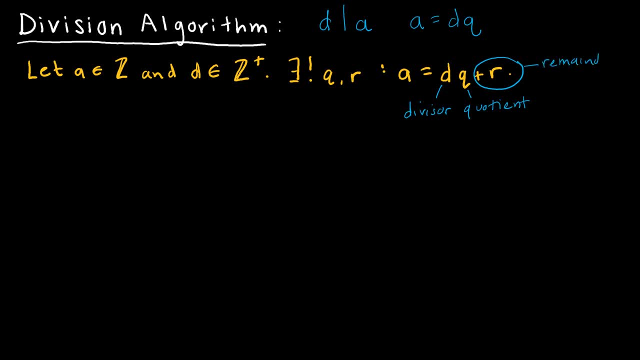 And R is going to represent a remainder. So let's take a look at an example on how we would use this. Let's say I want to see if 4 divides 21.. So 4 divides 21.. What this is telling me? 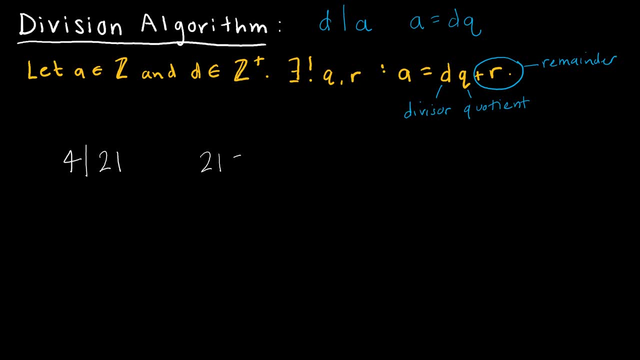 is. I can then rewrite: 21 is equal to 4 times some value plus some remainder. Now how would I figure out those values? Well, this is division. So let's kick it old school and say: let's say if I was putting 4 into 21.. 4 goes into 21 five times, which, of course. 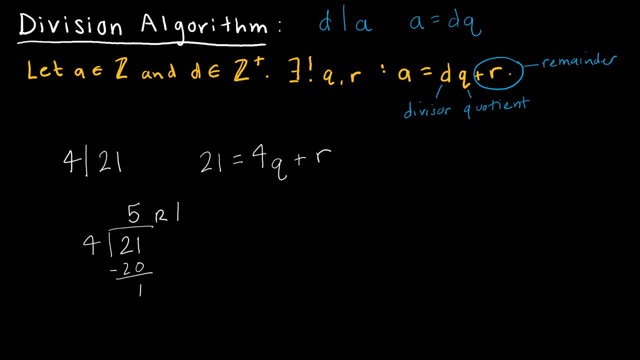 4 times 5 is 20.. So it would be 5 remainder 1.. That's all this is telling me. I can say: 21 is equal to 4 times 5 plus 1.. Now it's important when you're dealing with this that the remainder must be. obviously it could be 0. So it could be. 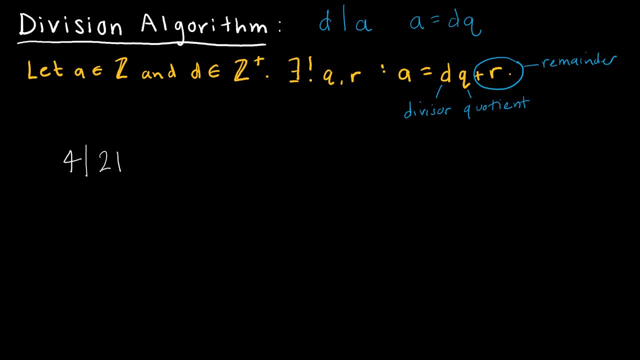 Let's say I want to see if 4 divides 21.. So 4 divides 21.. What this is telling me is: I can then rewrite: 21 is equal to 4 times some value plus some remainder. Now how would I figure out those values? 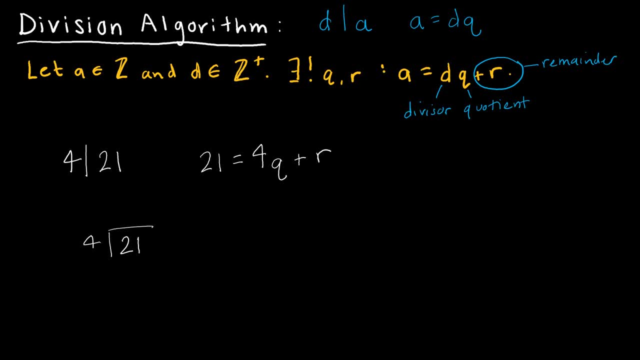 Well, this is division, So let's kick it old school And say: let's say if I was putting 4 into 21.. 4 goes into 21, 5 times, which of course, 4 times 5 is 20.. 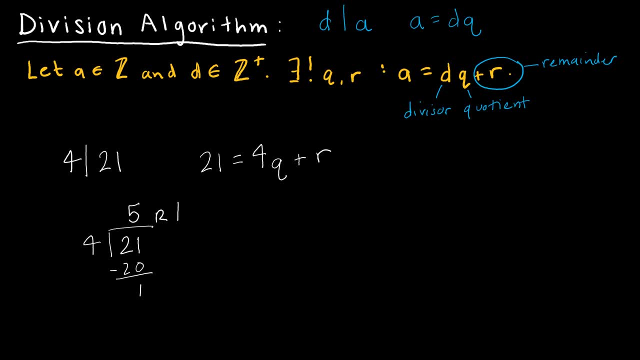 So it would be 5 remainder 1.. That's all this is telling me. I can say: 21 is equal to 4 times 5 plus 1.. Now it's important when you're dealing with this that the remainder must be. 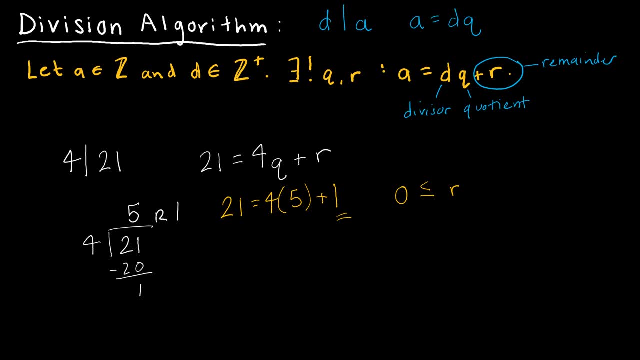 obviously it could be 0. So it could be equal to 0. But it has to be less than the divisor, And by that I mean if I said 21 is equal to 4 times 4, then my remainder would be 5.. 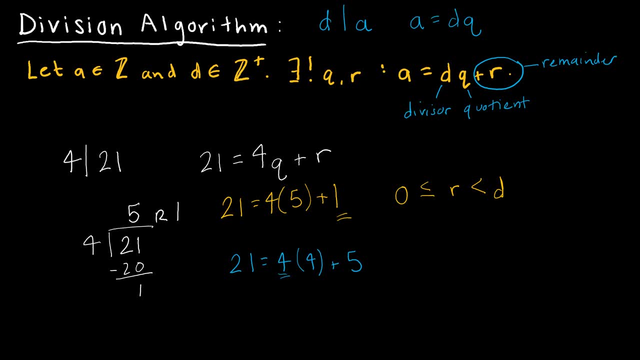 And 5 is actually greater than 4. And therefore I wouldn't want to use it because 4 could go in another time. So I've done this wrong. If this is larger than this, I've done something wrong. I would say, OK, well, I have to take one more of those. 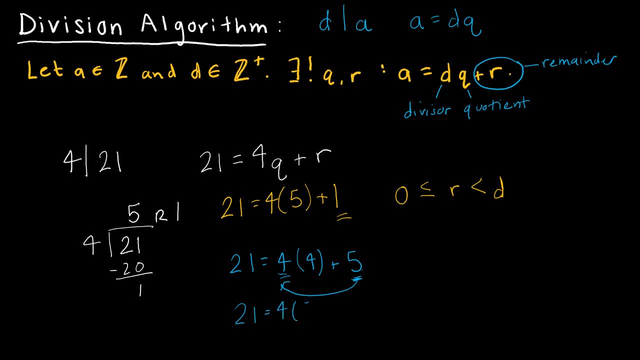 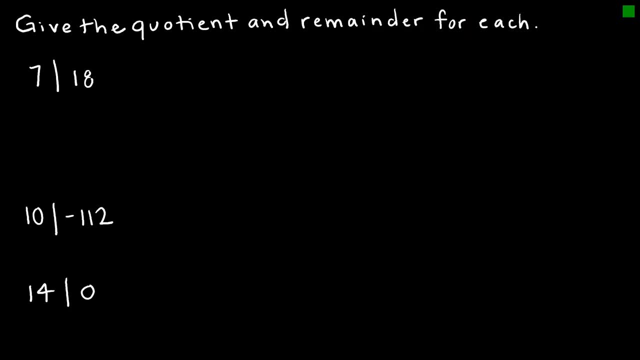 So 21 equals 4 times 5.. So this increased by 1. And this decreased by 4.. So let's take a look at a couple of examples here, using what we just learned, And remember what we just learned is A equals DQ plus R. 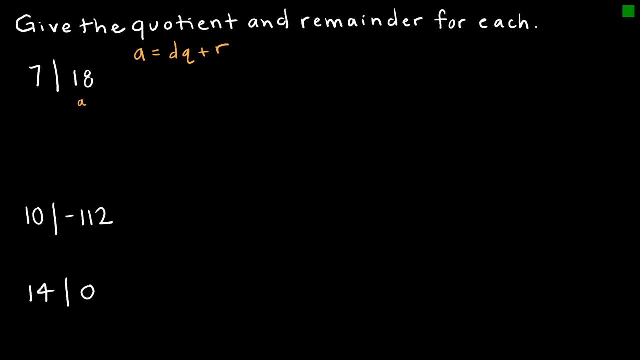 And in this case, of course, the A would be 18.. And the D would be 7, because we're saying 7 divides 18.. And so what we want to be able to do is we want to divide by 18.. 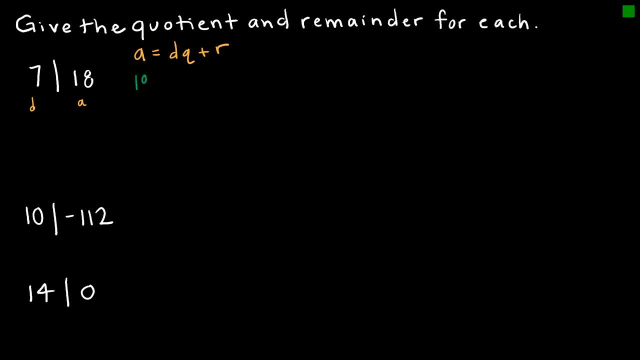 And what we want to do is we want to say that 18 is equal to 7 times some number, plus some remainder, And keeping in mind that R is between 0 and D, And D in this case is 7.. So all that means is the remainder has to be between 0 and 7.. 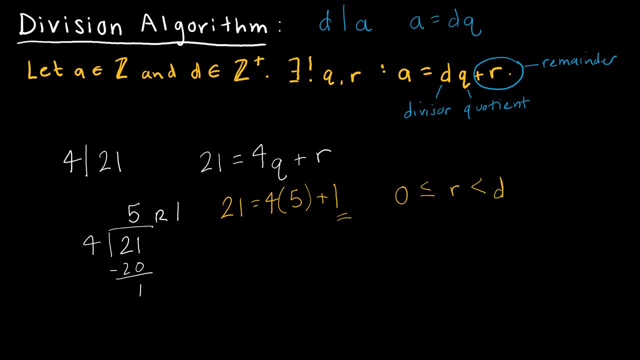 equal to 0. But it has to be less than the divisor, And by that I mean if I said 21 is equal to 4 times 4, then my remainder would be 5.. And 5 is actually greater than 4. And therefore I wouldn't want to use it because 4 could go in. 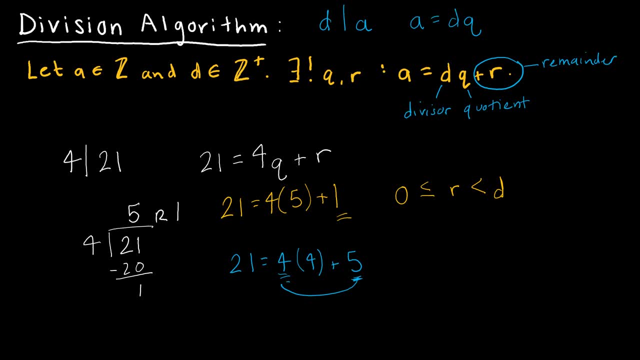 another time. So I've done this wrong. If this is larger than this, I've done something wrong. I would say, OK, well, I have to take one more of those. So 21 equals 4 times 5. So this increased. 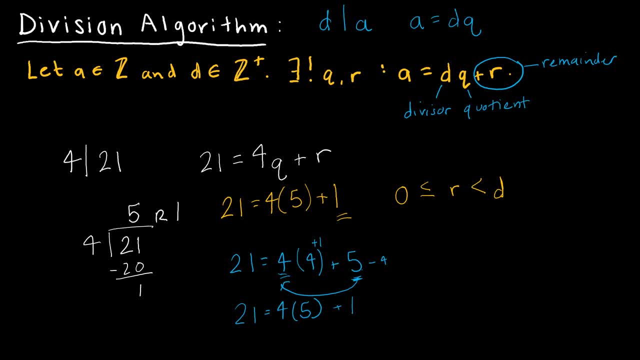 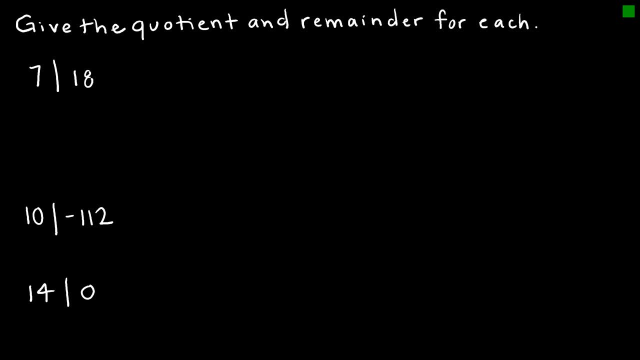 by 1 and this decreased by 4.. So let's take a look at a couple of examples here, using what we just learned, And in this case, of course, the a would be 18 and the d would be 7, because we're saying 7 divides. 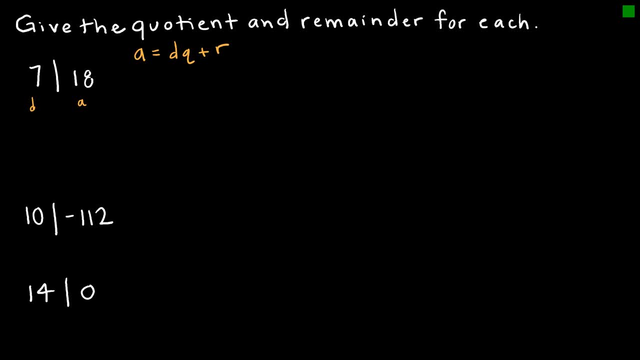 18.. And so what we want to be able to do is we want to say that 18 is equal to 7 times some number plus some remainder, And keeping in mind that r is equal to 7 times some number plus some remainder. 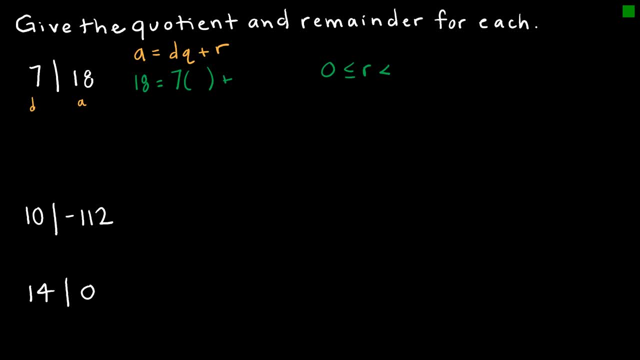 between 0 and D, and D in this case is 7. so all that means is the remainder has to be between 0 and 7. so 7 times 2 would give us that 14, and 14 plus 4 would give us 18. now I want to show you how we might write this as a quotient. oops, let. 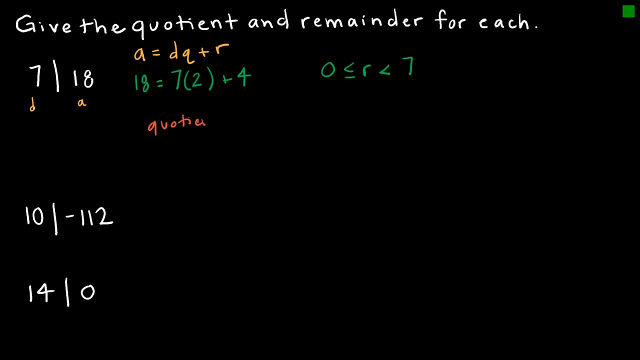 me try that again as a quotient and as a remainder. so this is maybe just a little bit different notation, just so you can see which will make will be very important to us moving forward. so a quotient can also be written as: Q equals a divided by D, and so in this case we're saying the quotient of 2 is equal to 18. 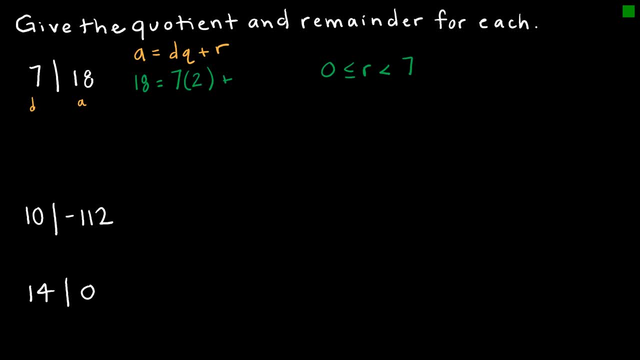 So 7 times 2 would give us that 14. And 14 plus 4 would give us 18.. Now I want to show you how we might write this as a quotient. Oops, Let me try that again As a quotient. 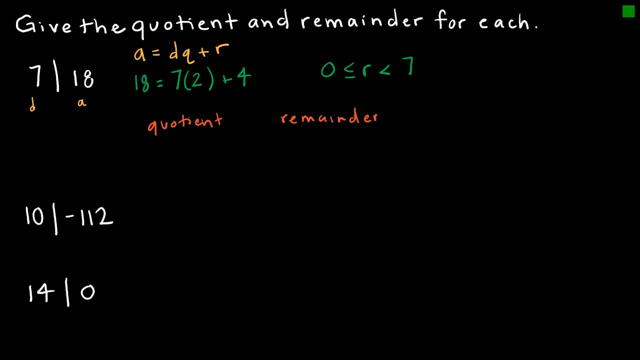 And as a remainder. So this is maybe just a little bit different notation, Just so you can see, which will be very important to us moving forward. So a quotient can also be written as: Q equals A Divide by D, And so in this case we're saying the quotient of 2 is equal to 18 divided by 7.. 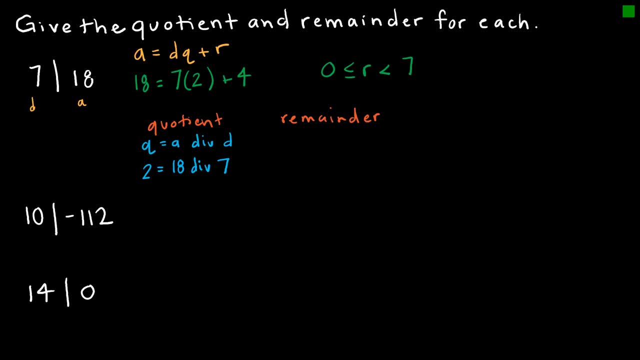 Which makes sense, because when we took 18 divided by 7,, 2 was the quotient. In order to write the remainder in the same way, we're saying: the remainder equals A mod D, So mod is sort of a new thing for us. 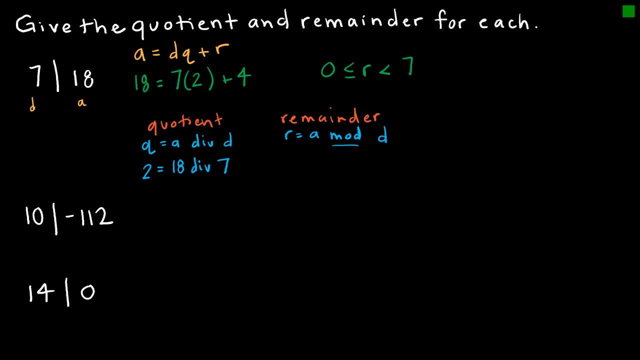 But essentially what we're saying is in a modulo of D, which is a base D number. basically we're saying if we divide A, then our remainder is A mod D. So in this case we're saying our remainder was 4.. 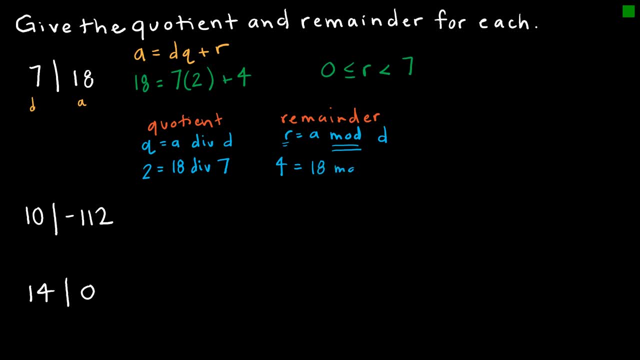 4 is equal to 18 mod 7.. And again, that just means if I took 18 divided by 7, my remainder would be 4.. Now the reason that I point that out to you is because in our next lesson, 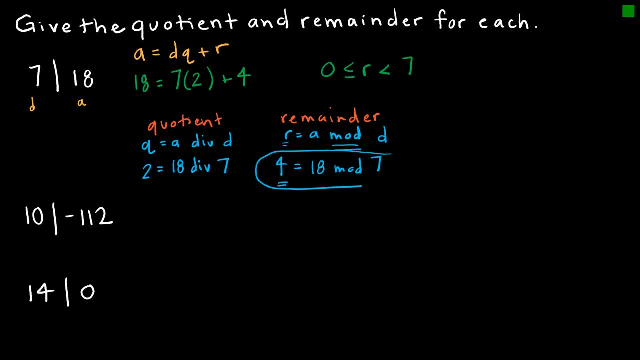 we're going to be looking at modular arithmetic And this concept right here is going to become extremely important to us. Now let's take a look at an example that involves some negative values. So again we're saying: negative 112 is equal to 10 times some number plus some other number. 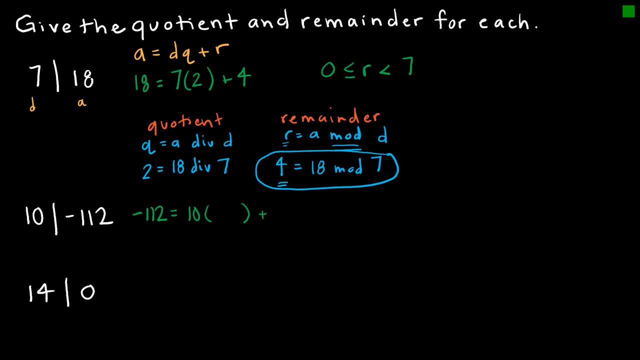 So this one's a little bit different. I could say: okay, 10 goes into 112.. That's 11 times, And if I took 10, I'm sorry that's negative 11 to make it the right sign. 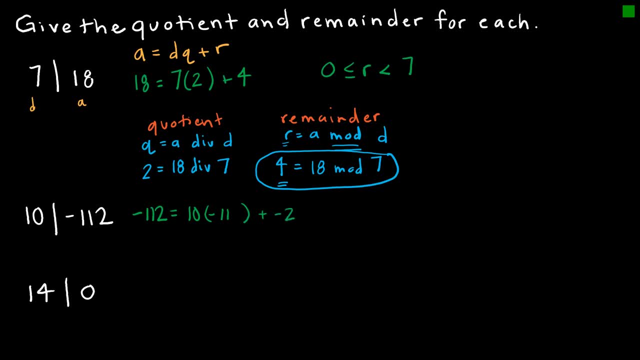 10 times negative. 11 is negative 110.. And then my remainder is negative 2.. But we know that my remainder in this case has to be between 0 and 10.. And negative 2 is not between 0 and 10.. 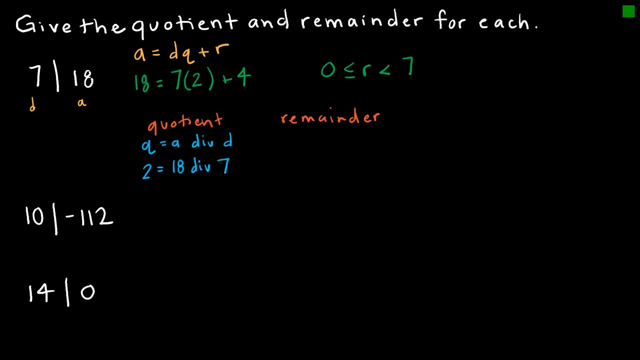 by D divided by 7, which makes sense, because when we took 18 divided by 7, 2 was the quotient. In order to write the remainder in the same way, we're saying: the remainder equals a mod d. So mod is sort of a new thing for us, but essentially what we're saying is in a modulo of d, which is: 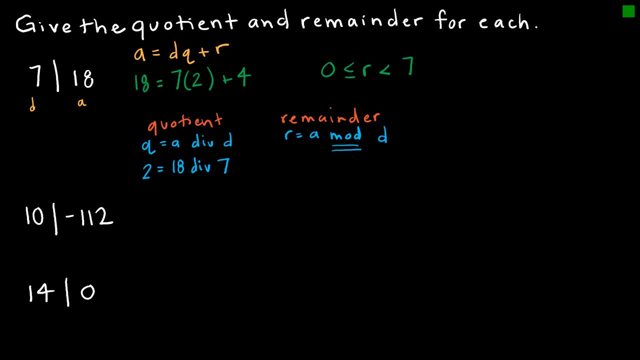 a base d number. basically we're saying if we divide a, then our remainder is a mod d. So in this case we're saying our remainder was 4.. 4 is equal to 18 mod 7.. And again, 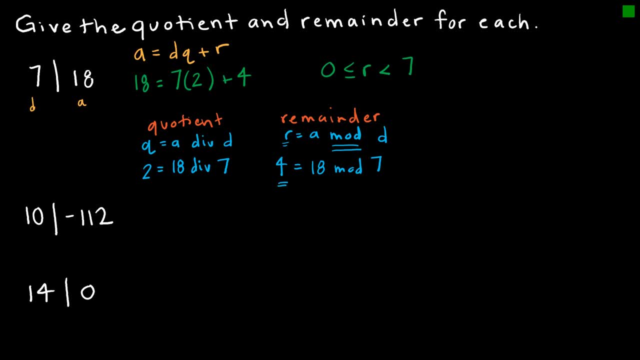 that just means if I took 18 divided by 7, my remainder would be 4.. Now, the reason that I point that out to you is because in our next lesson we're going to be looking at modular arithmetic, And this concept right here is going to become extremely important to us. 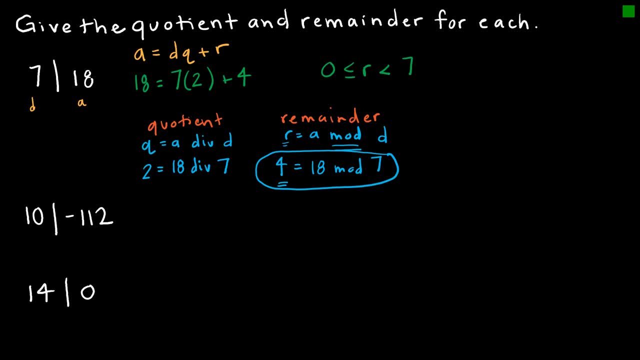 Now let's take a look at an example that involves some negative values. So again we're saying negative 112 is equal to 10 times some number plus some other number. So this one's a little bit different. I could say: okay, 10 goes into 112, that's 11 times. 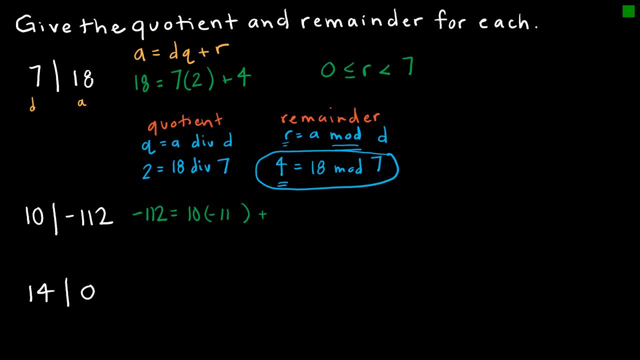 And if I took 10, I'm sorry that's negative 11- to make it the right sign, 10 times negative 11 is negative 110.. And then my remainder is negative 2.. But we know that my remainder in this case has to be between: 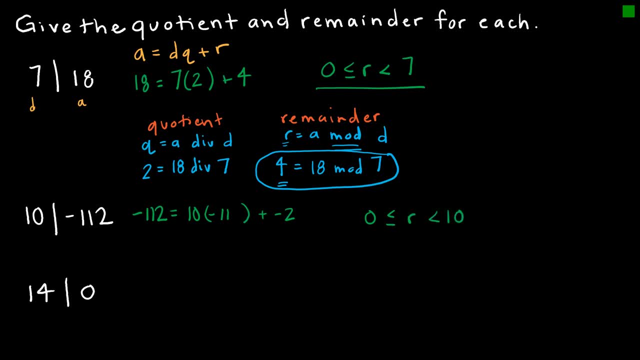 0 and 10.. And negative 2 is not between 0 and 10.. So instead of writing it in this way, I would have to write: negative 112 equals 10 times negative 12.. And then now my remainder is going to be positive. So if I took 10 times negative 12, that's negative 120,. 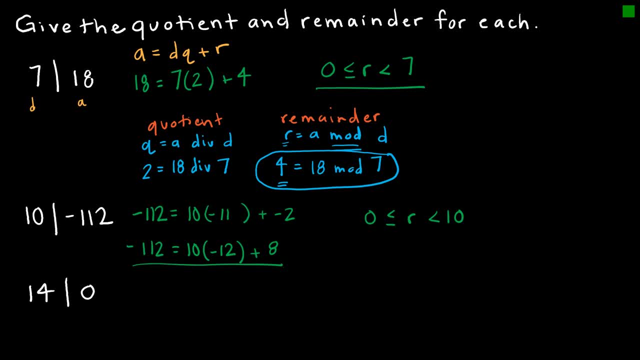 I would have to add a positive 8.. So this would be the correct way to write that. And then, of course, I need to write my quotient, which would be that negative 12,- oops, negative 12- equals negative 112 divided by 10.. 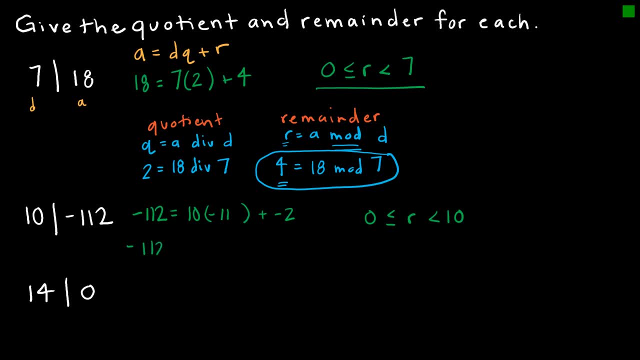 So instead of writing It in this way, I would have to write: negative 112 equals 10 times negative 12.. And then now my remainder is going to be positive. So if I took 10 times negative 12, that's negative 120. 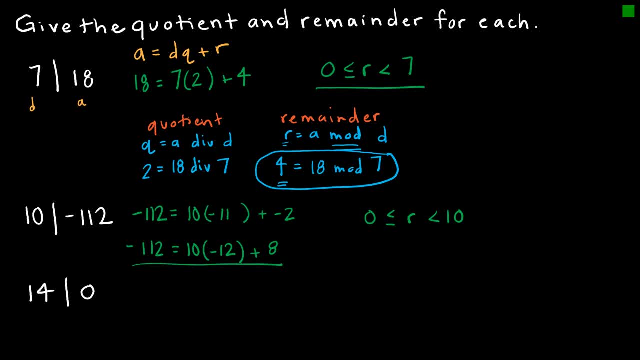 I would have to add a positive 8.. So this would be the correct way to write that. And then, of course, I need to write my quotient, which would be that negative 12.. Oops, Negative 12 equals negative 112 divided by 10.. 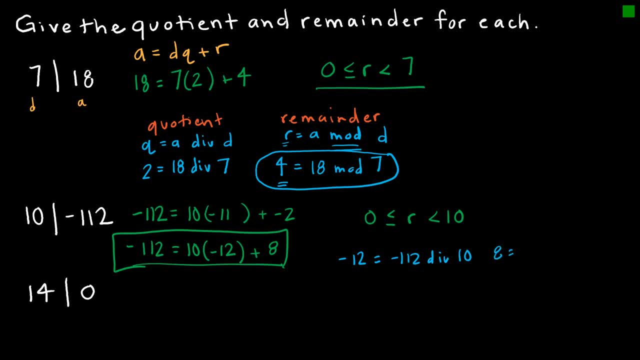 And then my remainder of 8 would be negative 112 mod 10.. And then our last one. This one's just a little bit different Because of course we are dealing with a 0. So essentially we're saying that 0 is equal to 14 times some number plus some number. 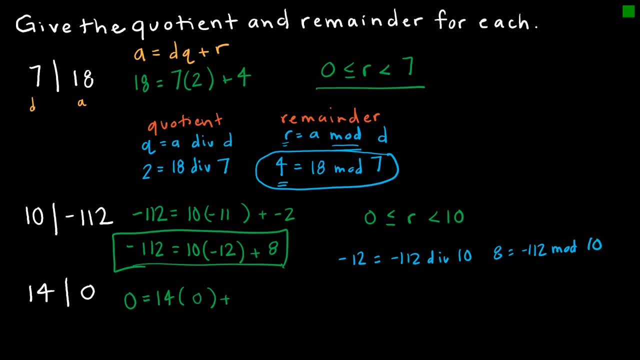 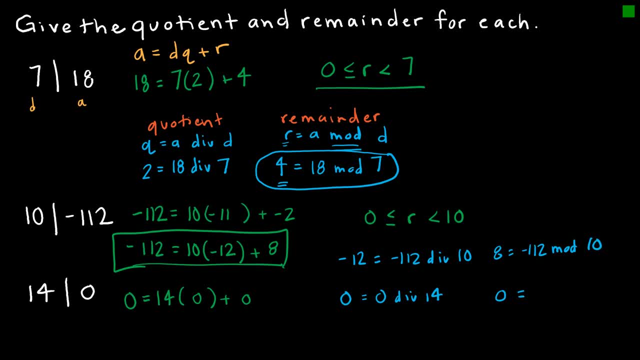 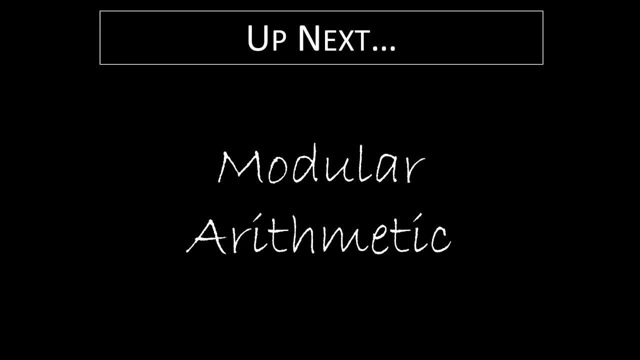 And that the remainder of 0 equals 0 mod 14.. Coming up next, we're going to take a look at modular arithmetic.